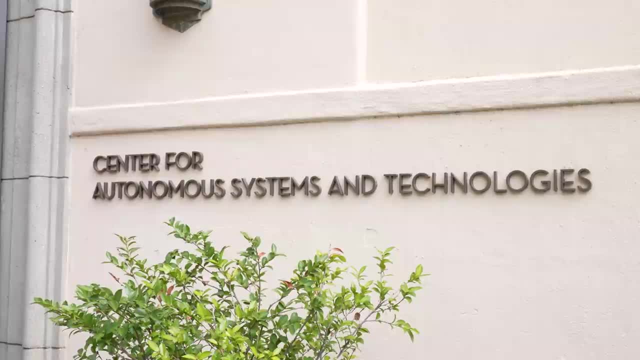 Good job. That is so cool to see. Yeah, Maybe. So the main facility for this lab is this one. It's a gigantic robot. It has a lot of weight. It has a lot of weight. So this one is a giant robot. 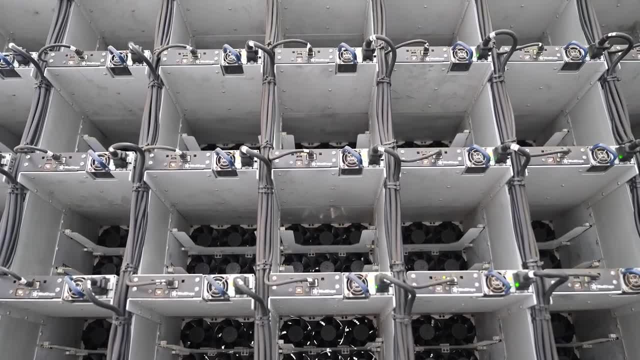 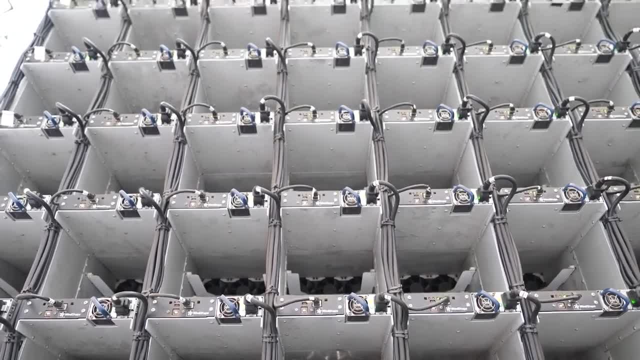 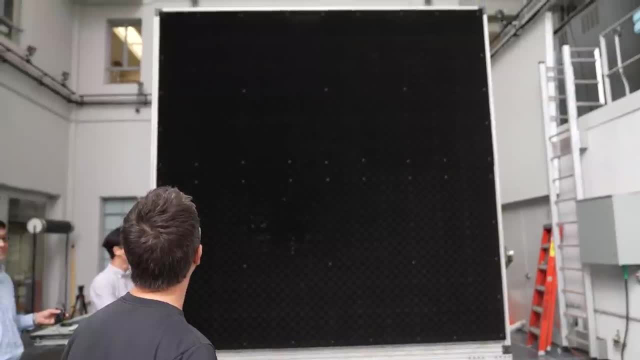 I can see all the fans now. Yeah, we have- you can't start counting- but 1,296 computer fans. Those are really literally computer fans. How fast can it generate wind? So up to 15 meter per second or 20 meter per second? 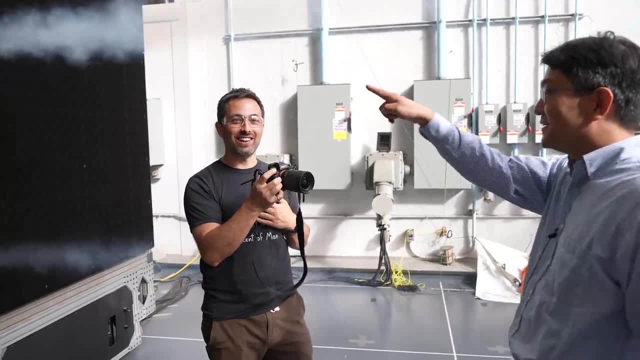 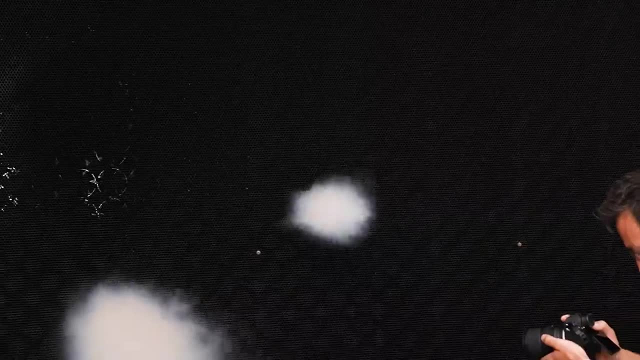 It's like a wind tunnel without the need for a tunnel. Yes, It might mess with our audio or with our microphones. Whoa, The idea of this smoke machine is to actually visualize the flow, but also with all these additional sensors like infrared cameras or radar and LiDAR. 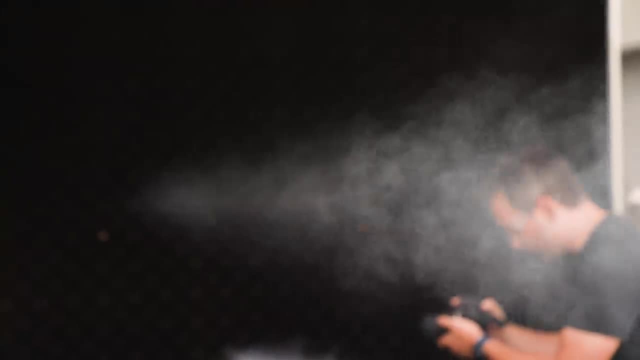 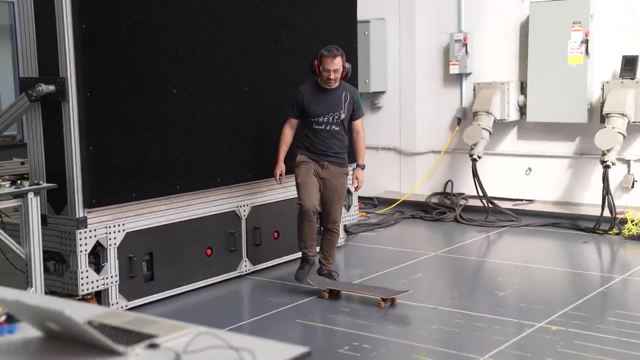 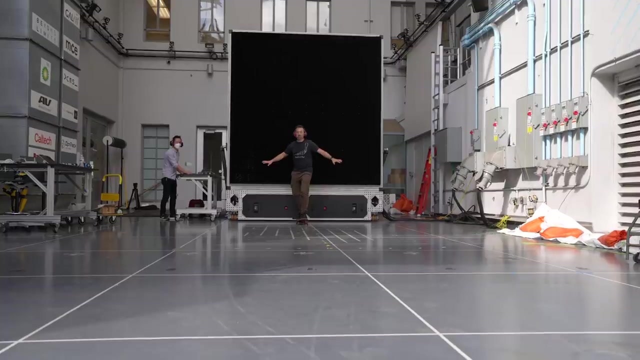 how we can actually figure out the kind of location or environment around your vehicle in the presence of this fog, And I wanted to feel their power for myself. All right, you ready? Yeah, let's do it. All right, That's a serious wind. 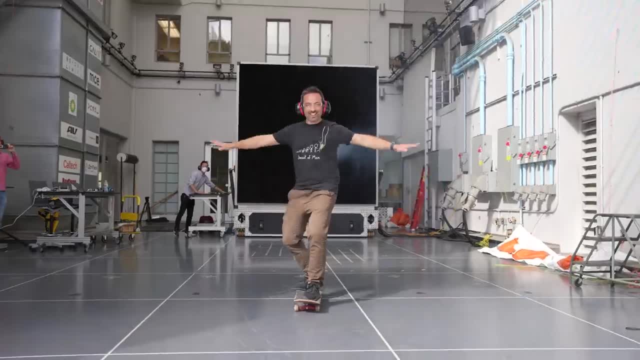 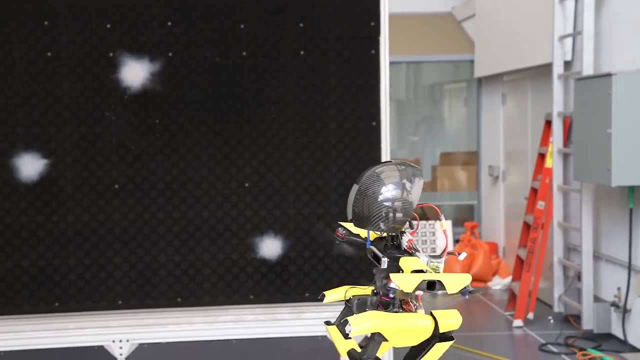 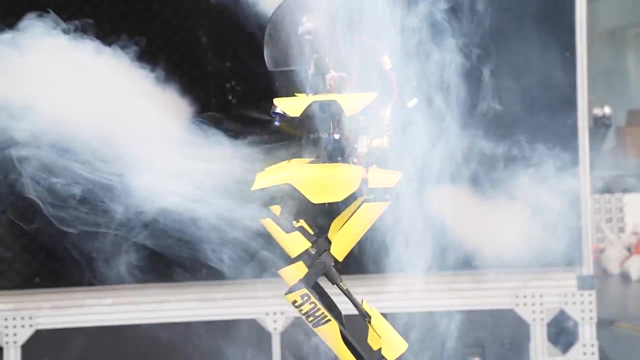 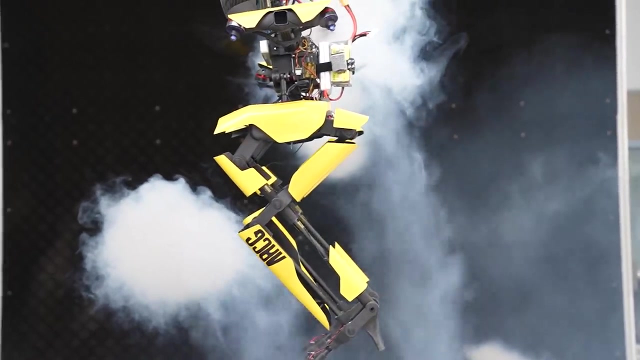 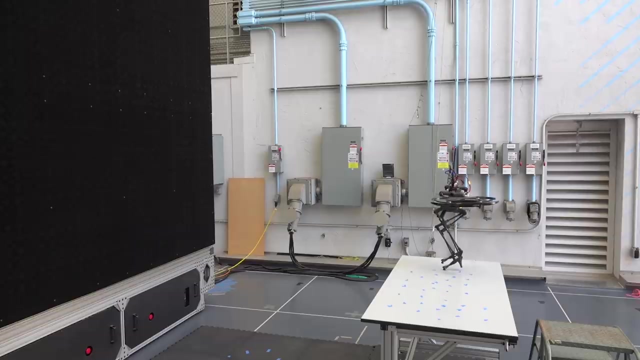 Ha ha. Yeah, That was so cool. I love it. They used this facility to test Leonardo to see how stable he is, even in different wind conditions, And we showed that LEO is more robust than a drone, because a drone gets blown away by the wind. 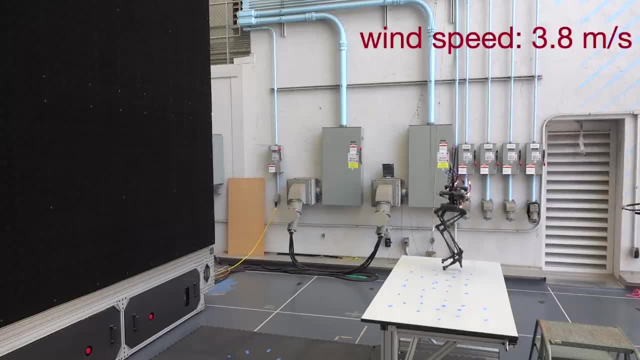 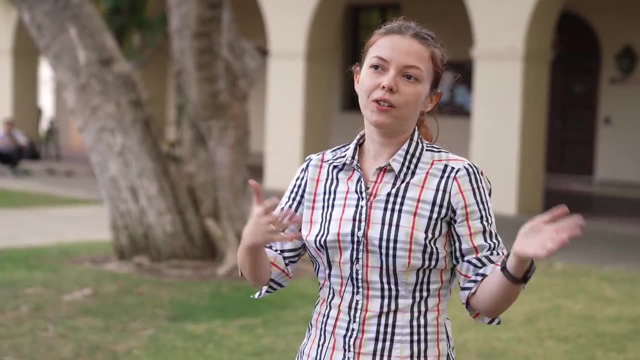 but then LEO does not because of its ground contact. So, for example, if you go hiking and there is like suddenly a lot of wind, you're not going to fall because you have the ground contact, But for a drone it might be blown away. 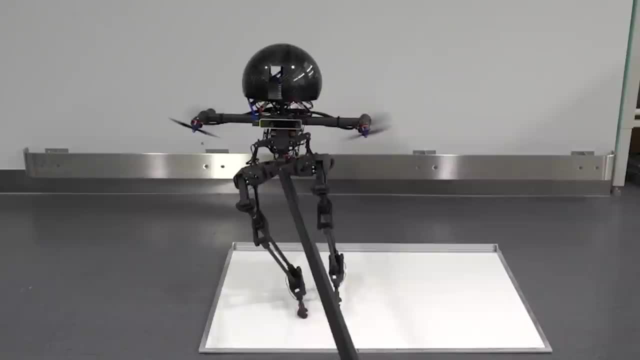 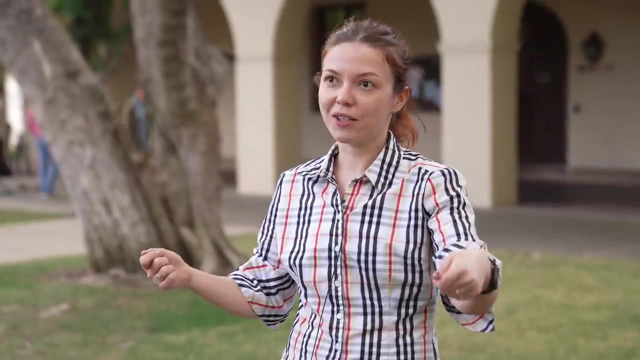 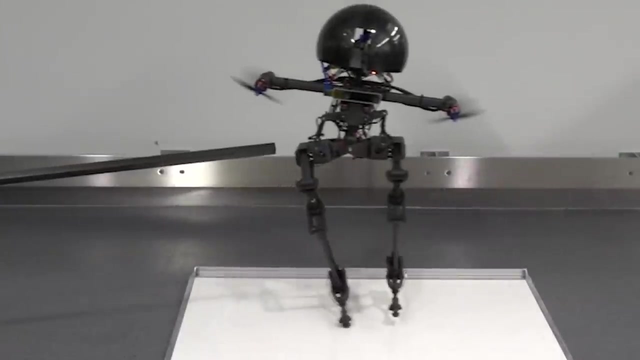 Oh no. So we actually took one of the whiteboards that we have at home and we put oil, So we applied perturbations to LEO And what's happening is, as you push LEO, instead of falling it stays upright, but it also slides on the whiteboard. 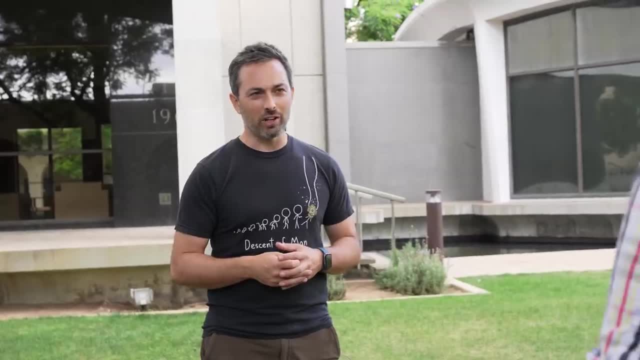 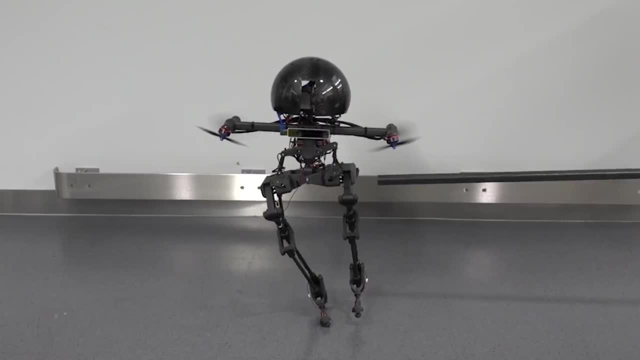 So that's an interesting capability, So it's very robust. You said perturbations. Are you poking the robot? Yes, Without harming the robot. we are gentle. Leonardo is so stable and good at adjusting its balance that it can skateboard. 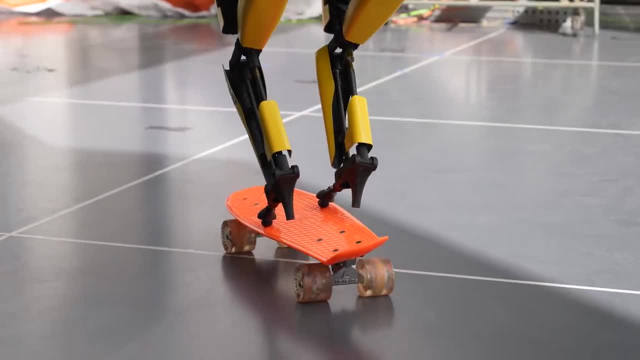 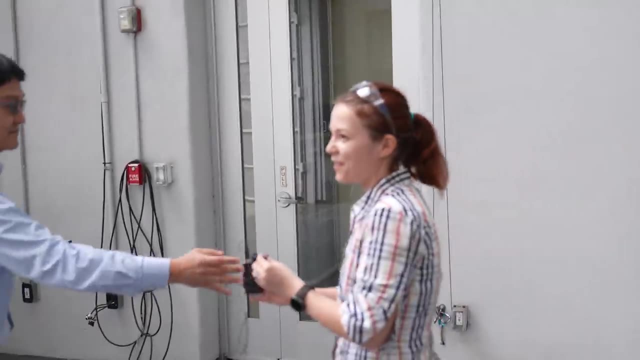 That's a fancy trick. Not many people can go backwards on a skateboard. How did you get the idea for a robot that will skateboard? Should I say the truth or make a nice story? Tell us the truth. Yeah, so we went hiking and we saw about 10 people going. 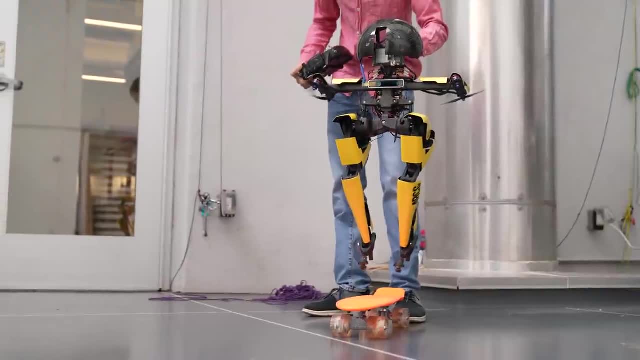 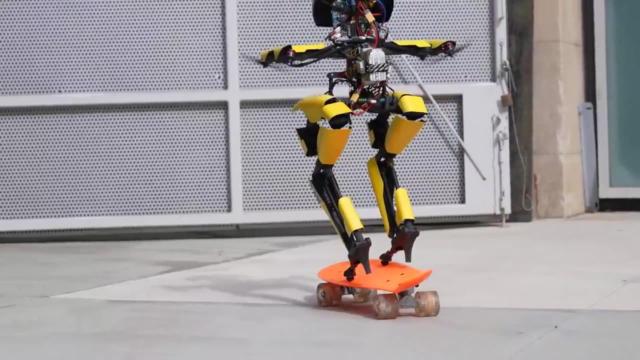 down the mountain on a skateboard. and then we thought, wow, this is really cool. What if we try our robots to make it do this? So we went to the first shop and we bought a skateboard, We modified it and we tried it and it worked. 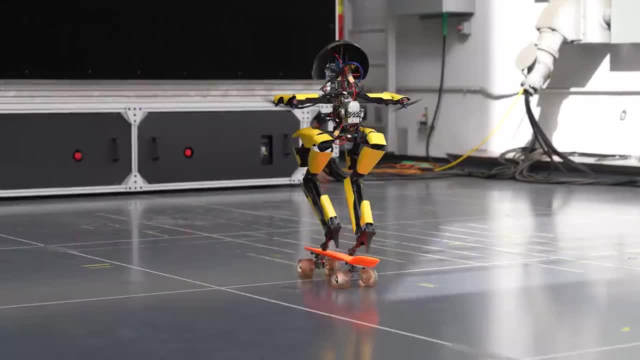 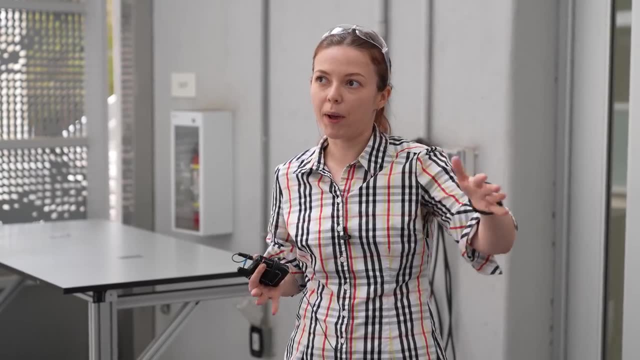 So do you think it allows the robot to save energy by riding on a skateboard? It's more efficient because it uses the legs less. The legs are basically used to steer, and then it's just the propellers that I use to accelerate the skateboard forward. 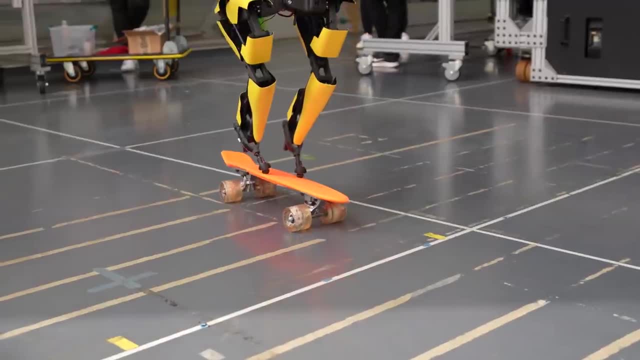 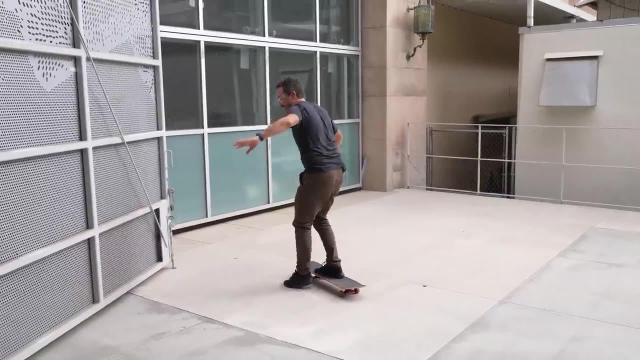 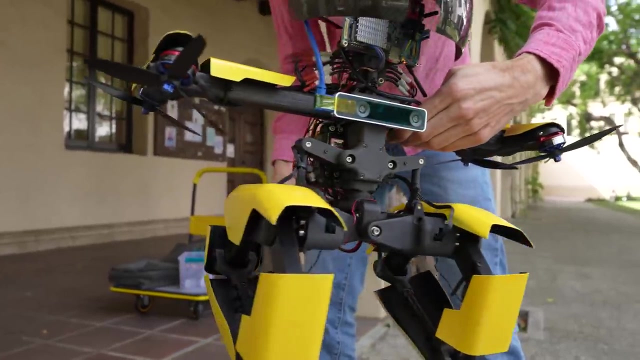 and backwards. so, yeah, it makes it save a bit more energy. The propellers, of course, make it possible to skateboard backwards, something I struggled with. It definitely would help if I had a propeller, But the real challenge was slacklining. 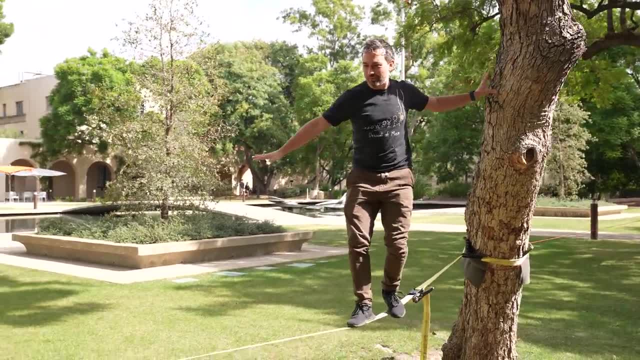 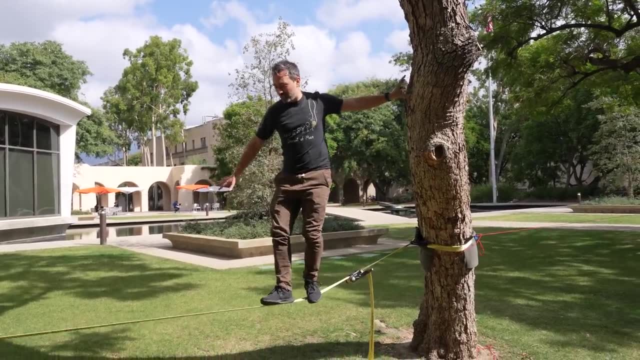 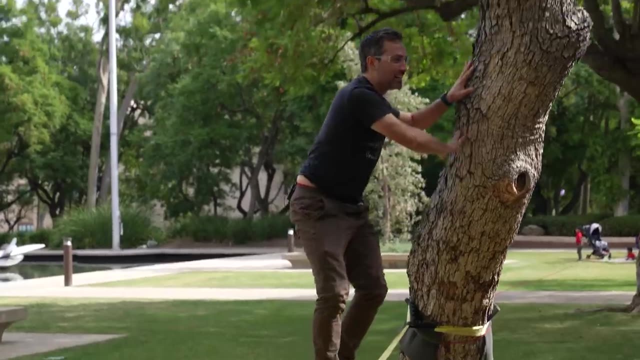 This looks incredibly unstable, so I think this proves the point of just how important control systems are. You can tell from the footage. I have no idea what I'm doing. All right, I thought I would be slightly better at that. Let's give it another shot. 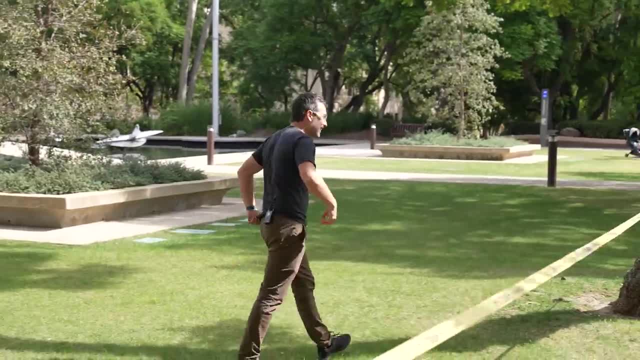 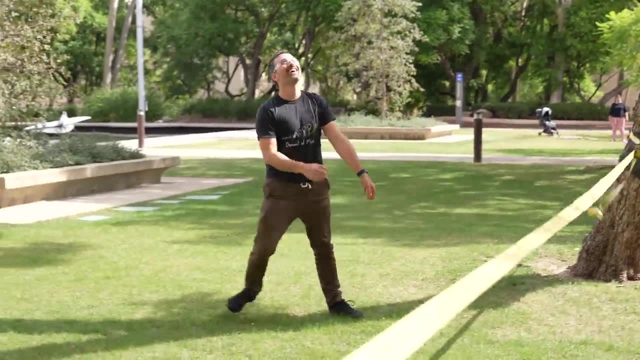 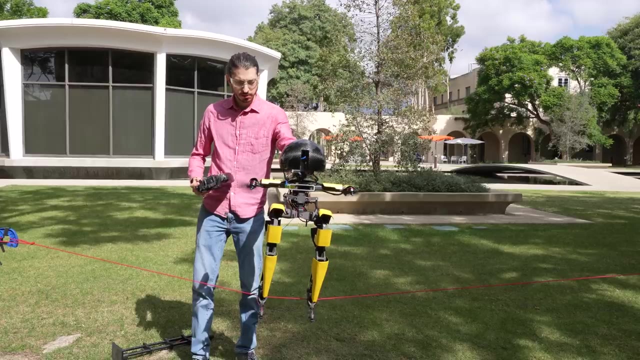 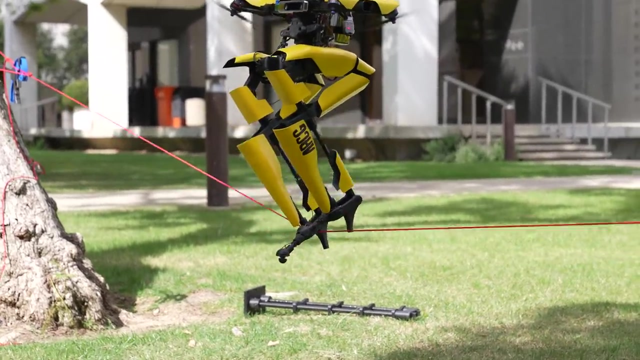 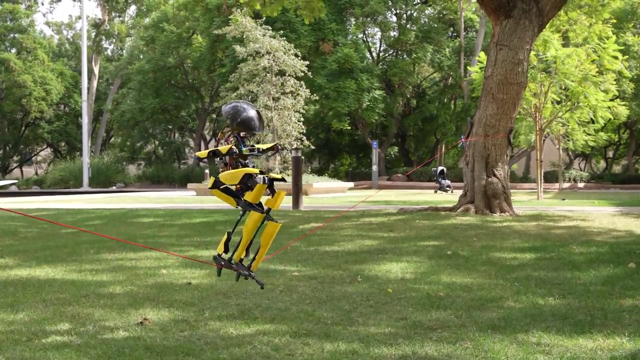 OK, Can anyone slackline? This is impossible. I need a robot to do this for me. I'm just going to между and turn around for one second. I like the side-stepping technique. Maybe I should have been doing that. 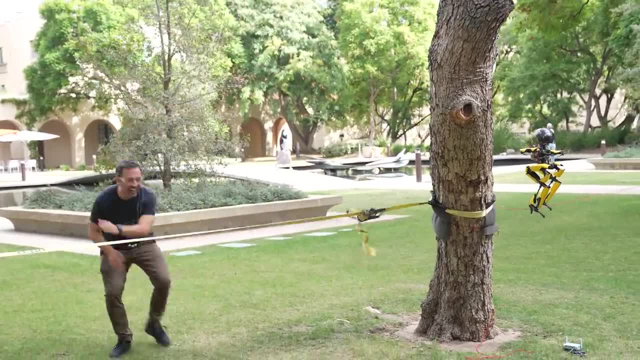 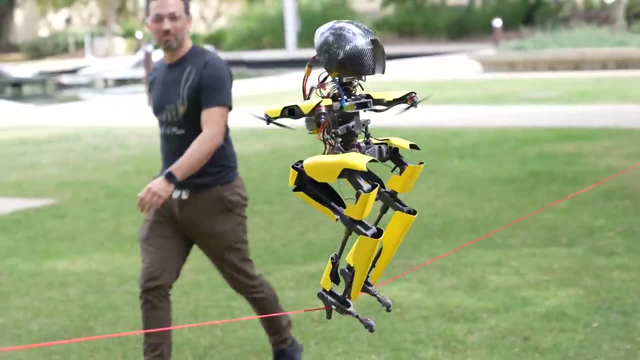 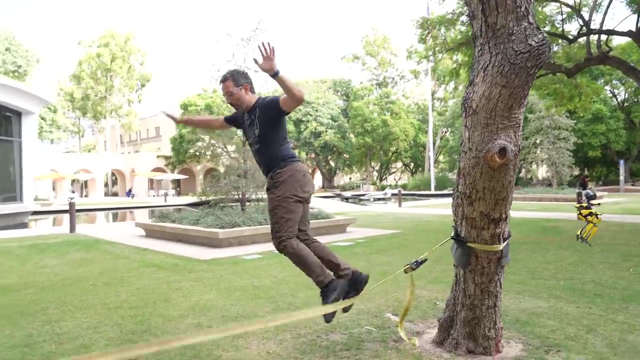 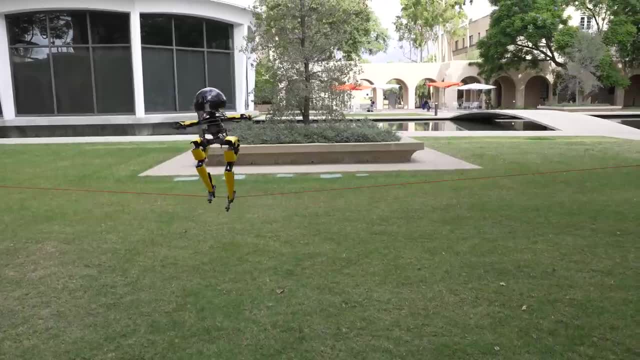 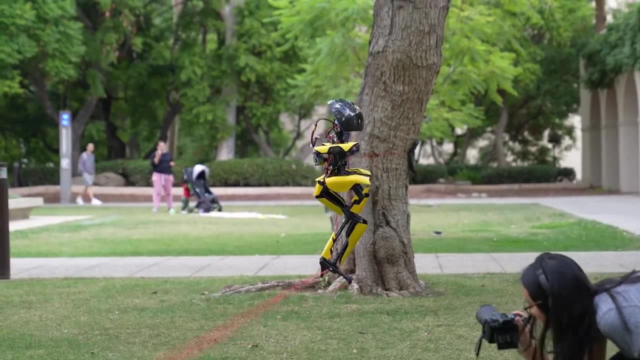 I should've prepared. You might think it's cheating to use propellers, but the robot is clearly not flying. It is supporting itself, mostly using the rope, and it's able to stabilize itself even with the wild bouncing. So human professional select liner. 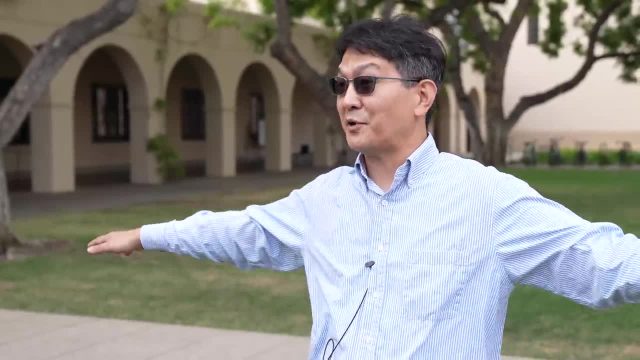 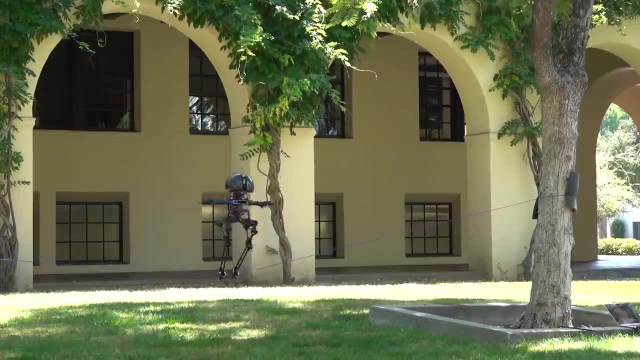 if you see some of their videos. actually they use the arm stretch and then they can balance themselves. We don't have the arms for Leo yet. We are planning to add the manipulation so that it can actually carry some object, But in the meantime we are using the propellers. 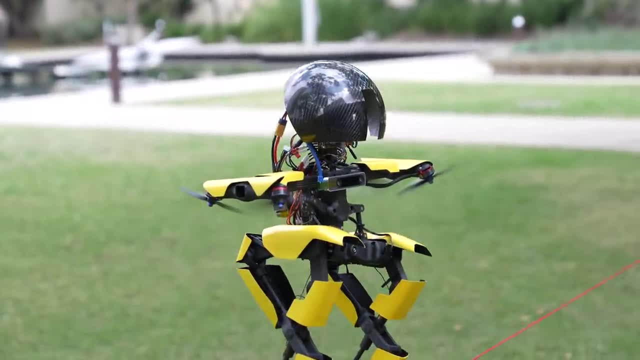 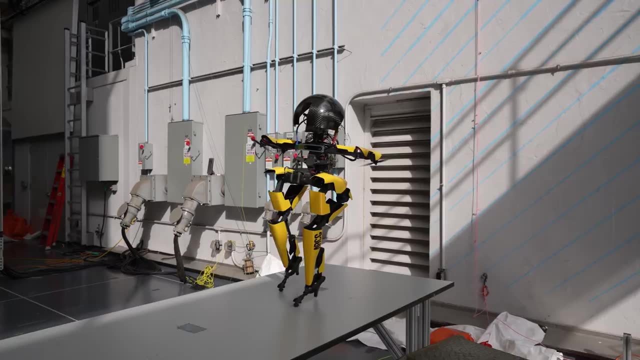 to stabilize the Leo, while it's actually walking on a select line. It's funny because the robot feels like it's got kind of a personality to it the way it walks and flies. Yeah right, It's just totally something you're not used to seeing. 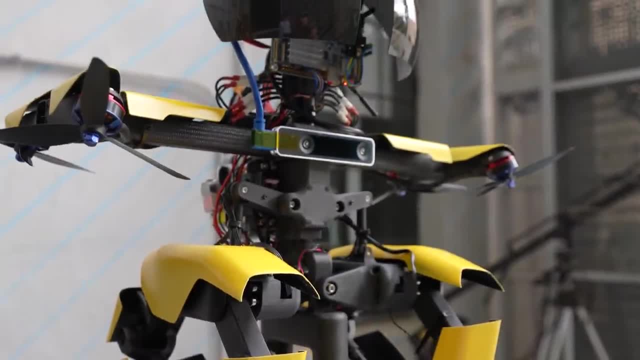 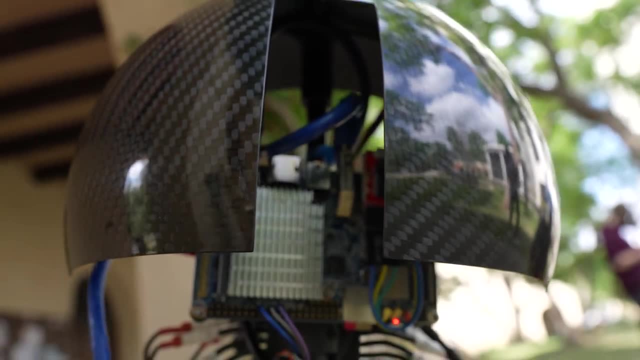 Yeah, it looks natural. Actually, I have to say that the sensors are sampled at 1,000 times per second, But the controller is actually being recomputed, whatever signal you are sending to propellers and the leg joints, 200 times per second. 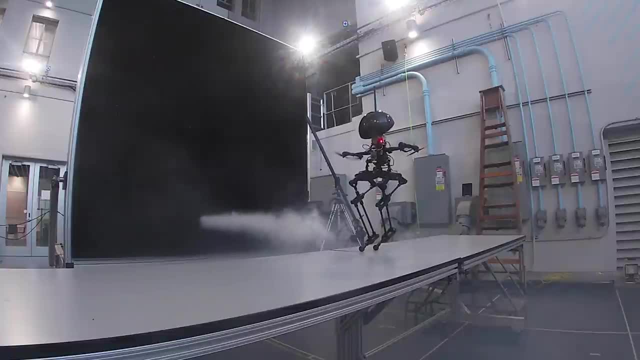 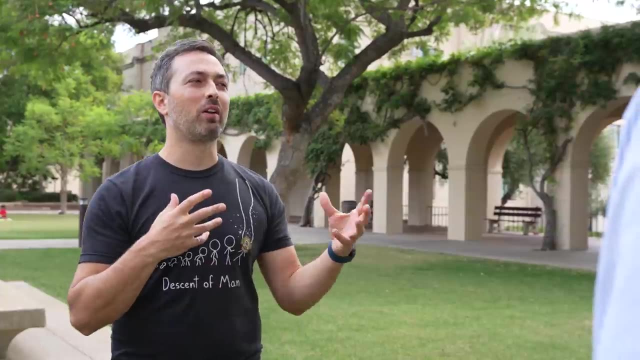 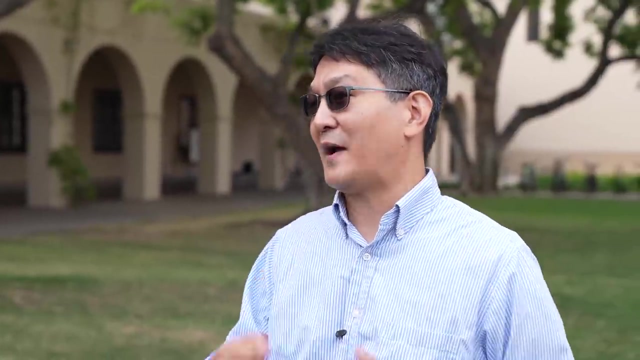 So it's a pretty fast computation: 200 times a second. it is adjusting what it's doing to maintain balance. Yes, especially propeller control signal. How does that compare to humans? Humans? So humans can do very sophisticated tasks, But in terms of fast reaction it's a very crude machine. 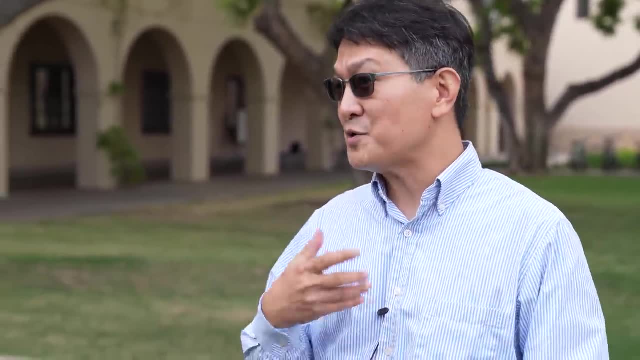 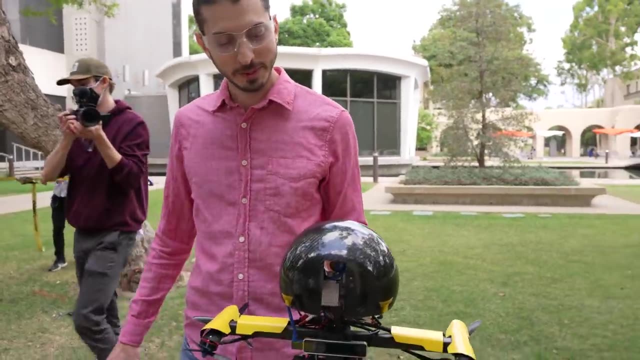 So humans, in fact, can overall, have a few seconds of delay, time delay. Is this why I was struggling on the slack line? Maybe, but How do you feel about the performance here today? Yeah, I think it beat you. 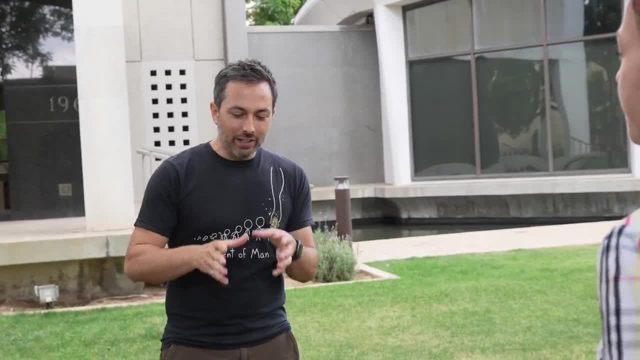 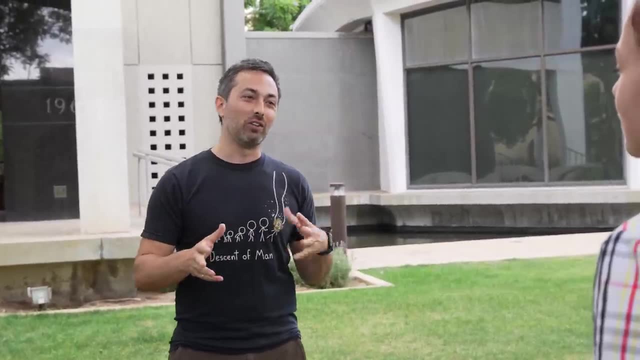 I mean not that that's hard, but this is very impressive. If you imagine a robot like Leonardo in the future, like the greatest Leonardo you could make, what would that robot look like and do So? definitely having a Leo-like robot in space. 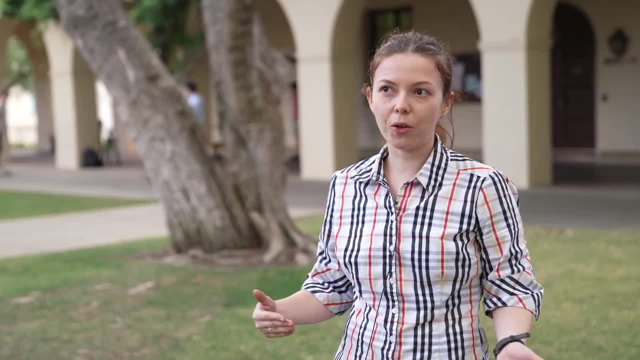 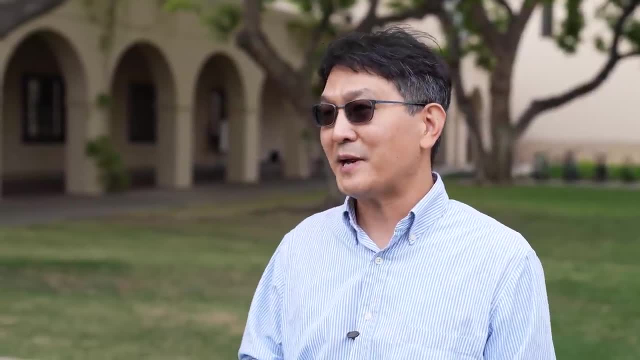 that would be amazing, But of course, depending on where you go, you might not be able to use propellers, so then you would need to use thrusters. So eventually, yes, we want to develop this lag-based adaptive landing gear. 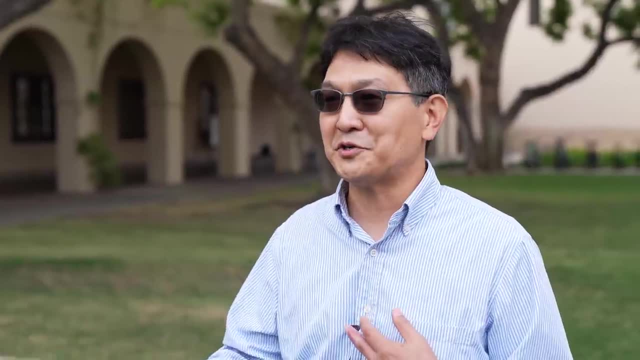 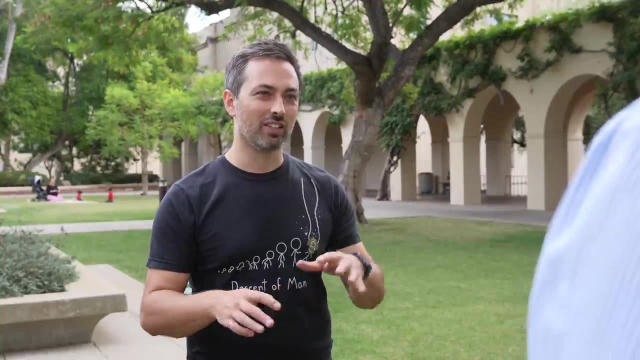 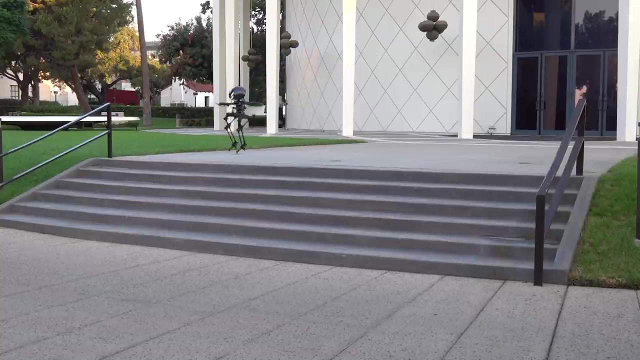 and then we give that to next generation Mars helicopter or next generation flying cars so that it can actually land in very challenging conditions And still move around once it's on the ground. Yeah, once you land, then you can walk over it. Imagine if you have a robot. 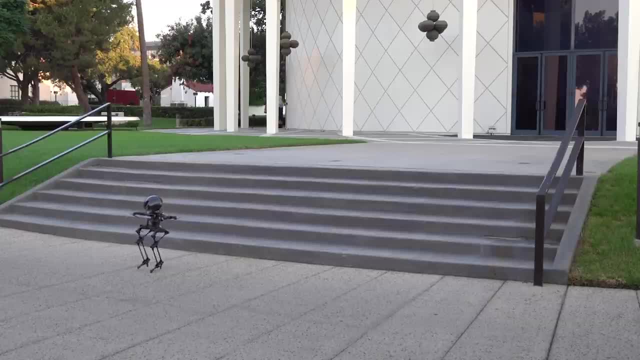 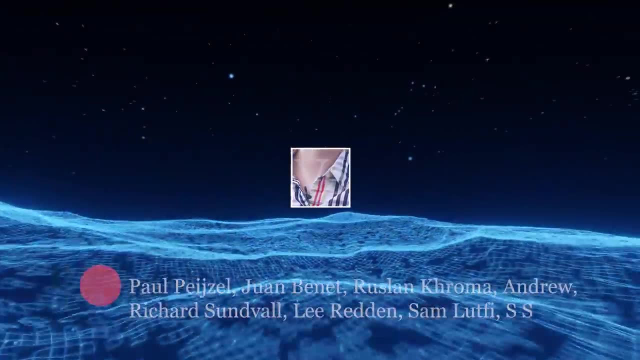 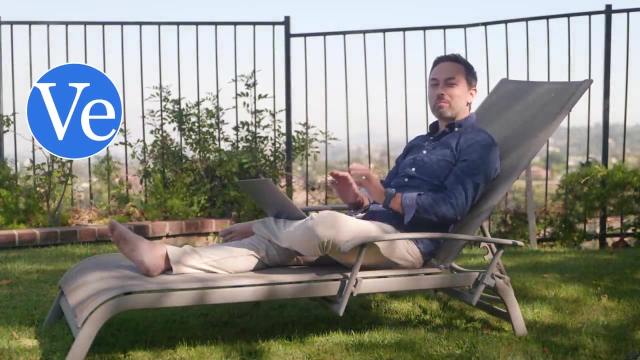 have a cliff and then you have the robot: just jump out of the cliff, deploy the propellers and fly. That'd be wild, Oh hey there. This portion of the video was sponsored by Bluehost. You know, tech is now so advanced that robots can skateboard, So why is it still so hard to 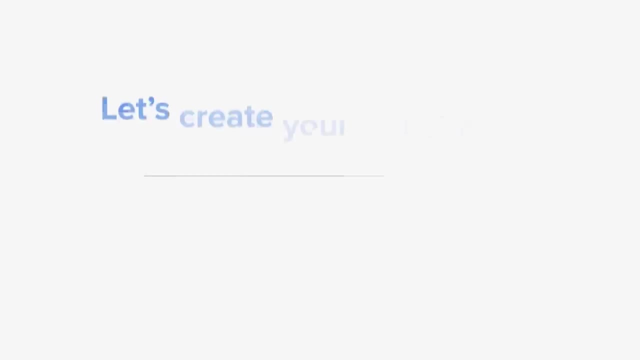 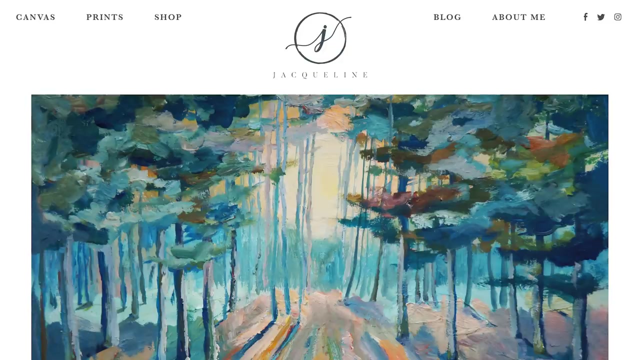 build a website. Make the process simple. with Bluehost, It's easier than ever to get started. Bluehost provides you with a completely free domain for the first year, as well as quick start templates, So you can have a beautiful website up and running in just minutes. The 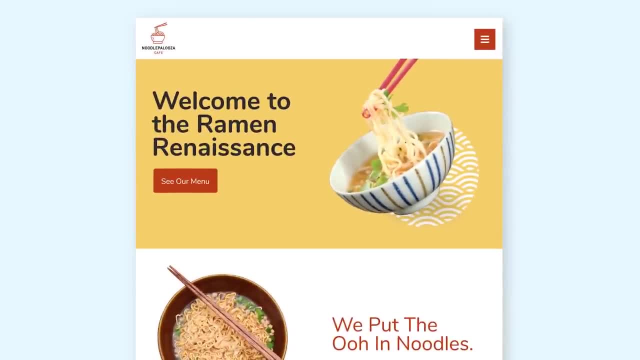 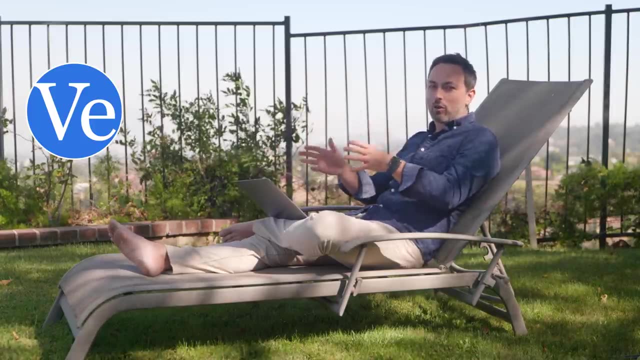 templates are mobile ready, So your website is optimized for both phones and computers from the start. Unlike the process of building a robot like Leo, you don't need code in order to make your website. Bluehost lets you customize everything with simple drag and drop editing. 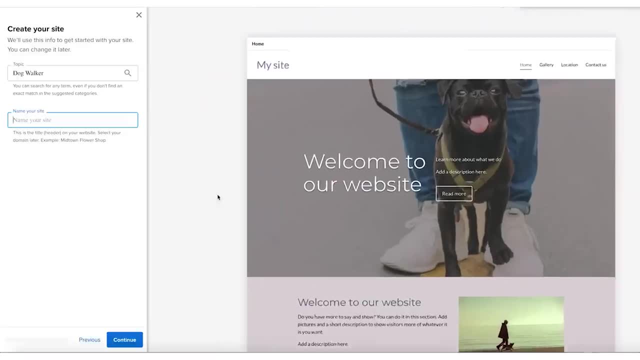 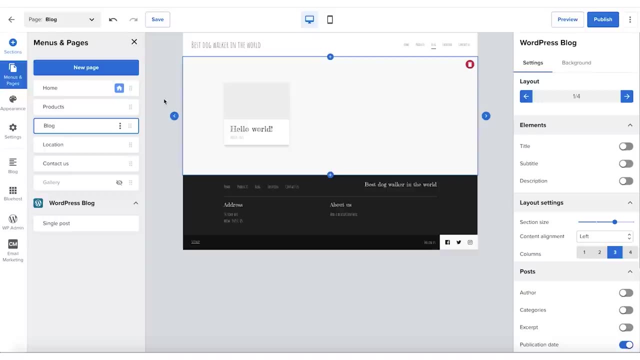 And Bluehost builder also allows people to choose their own editing journey. It's built on WordPress, So at any time you could toggle between WordPress core, the traditional editing experience, and the Bluehost builder with no loss of functionality. This is a first of its kind builder experience, So start building your. 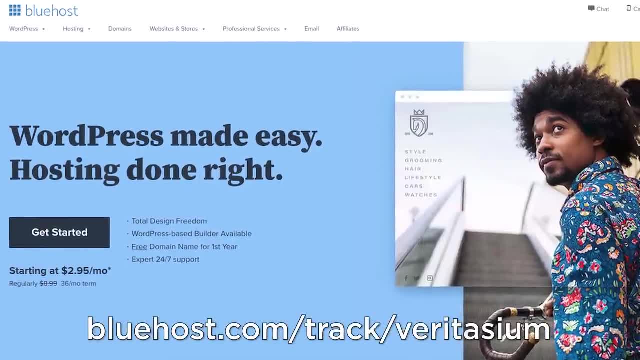 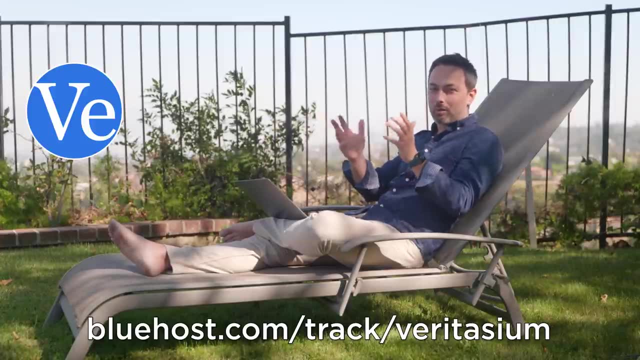 website today with Bluehost. Just go to bluehostcom slash track, slash veritasium to receive more than 65% off. I will put that link down in the description. So I want to thank Bluehost again for sponsoring this portion of the video And I want to thank you for watching.